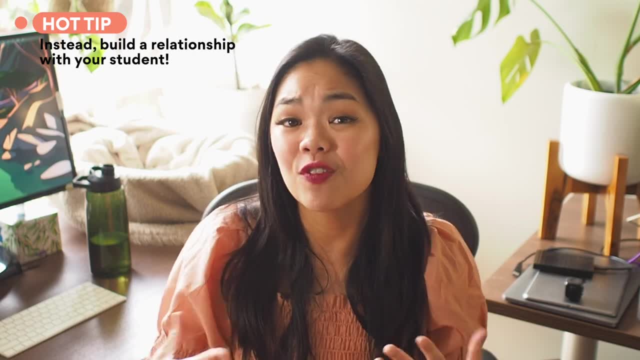 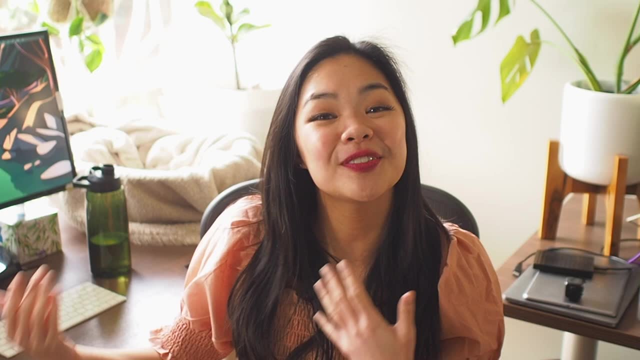 with your student When it comes to tutoring. it's a unique experience, And if you've had tutoring before, you know what it feels like- in that you can get quite close to your tutor. They're that person that you see week after week. They really get to know you in terms of your studies, but they 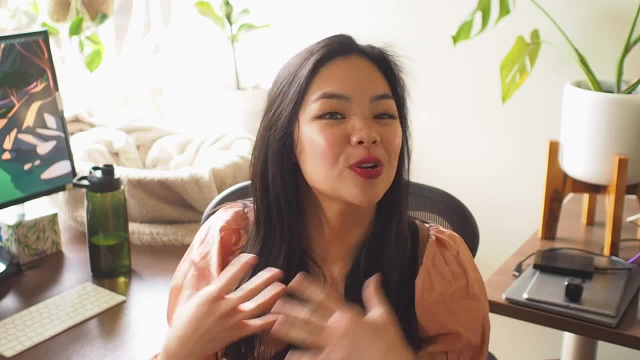 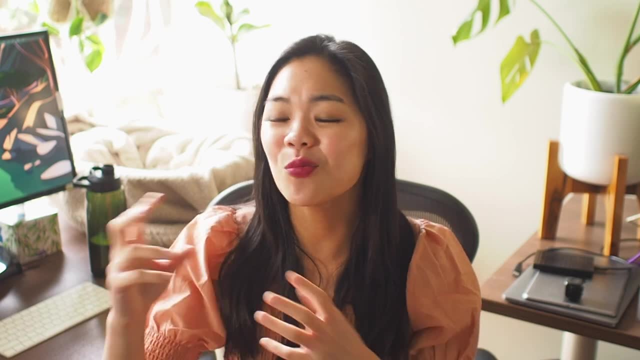 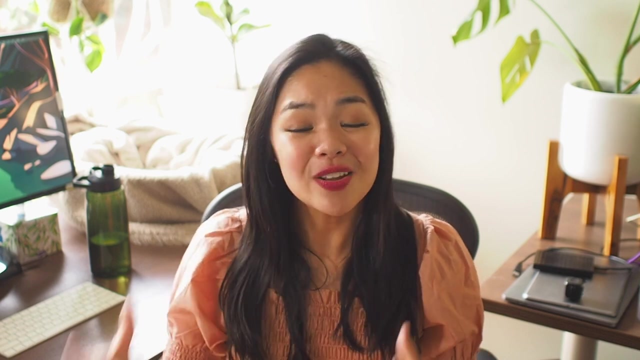 also get to know you potentially as a person as well, because they get to understand what your motivations are. They get to know you week to week leading up to exams, how stressed you are, what else is going on in your life. It can be often a therapeutic session for a lot of students, So the benefit there. 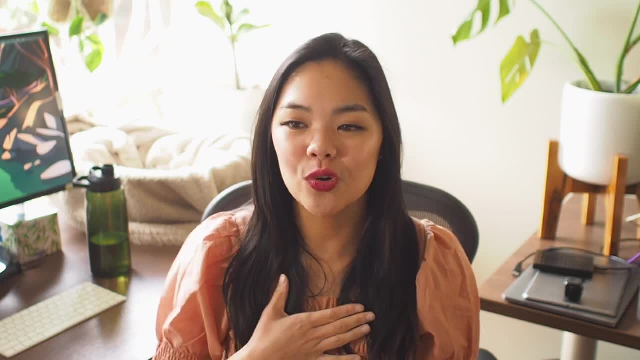 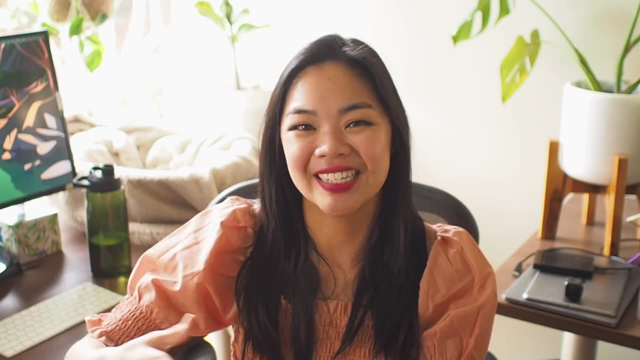 is that it's actually really nice for tutors as well, When you know that you're not just there just purely for that expert knowledge, but that you can support them in just general life advice and life mentorship. Let me know in the comments below, by the way, if you've had this experience. 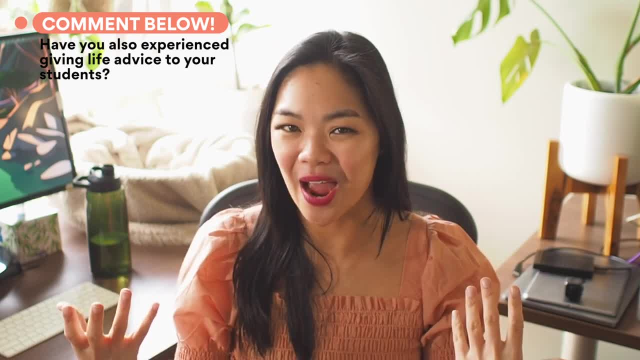 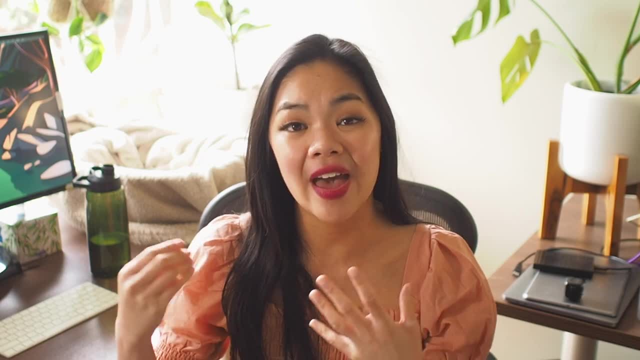 as well, or whether or not it's just me and the tutors that are watching this video right now that I work with And the added benefit of building that relationship with your student and taking the time to do so means that you both have a better tutoring experience. They feel safe. 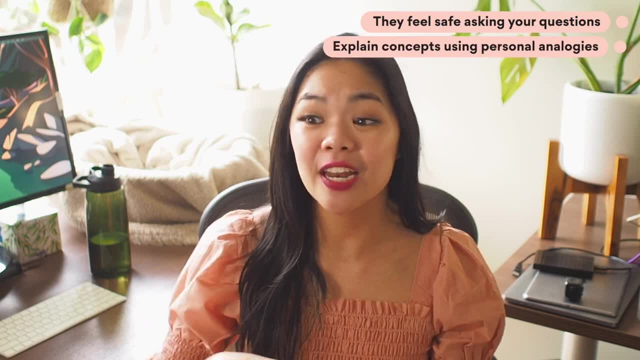 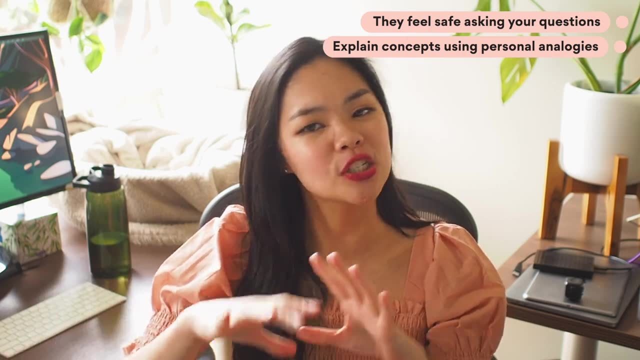 asking you questions. If there's a concept that they don't quite understand, you could take aspects of their own personal life and use that as analogies as a way to explain things. There's just an array of benefits that happens once you actually build that relationship with. 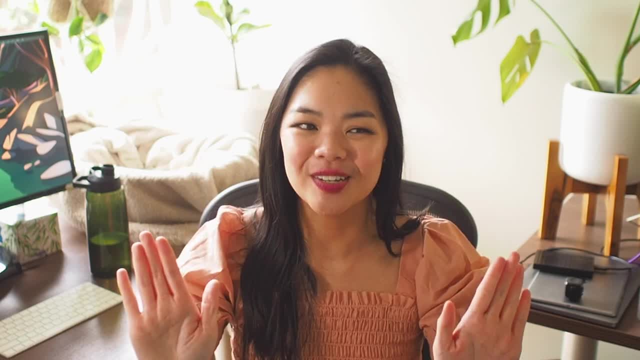 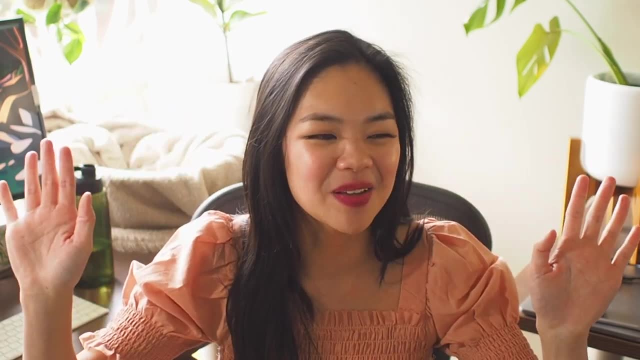 your student And I just want to clarify- I know this is obviously a very popular and student relationship- We're not talking about romantic relationships. I don't know if I need to disclaim that, but I'm just going to put it out there anyway. So different. 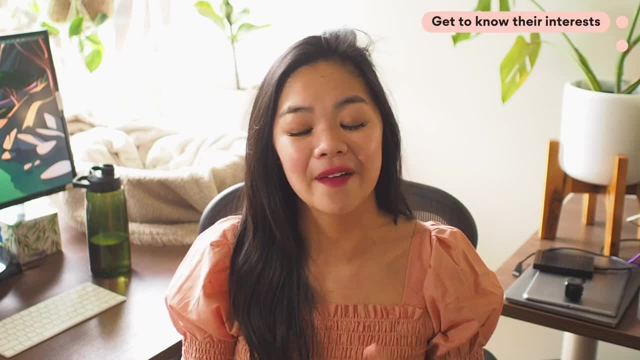 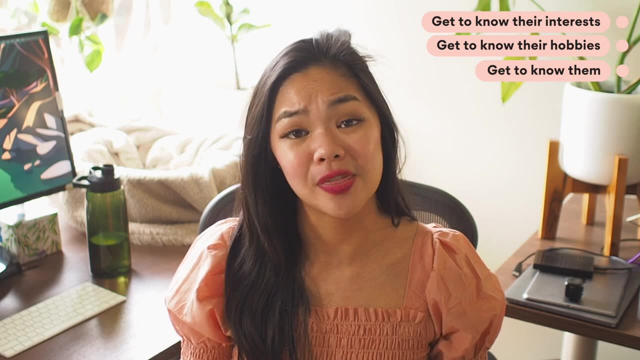 things that you can talk about. you can talk about what their interests are, their hobbies, get to know them as a person. basically, It's as simple as that. You'll find that the value they get out of the sessions will be a lot more than if you just bombarded them with knowledge. 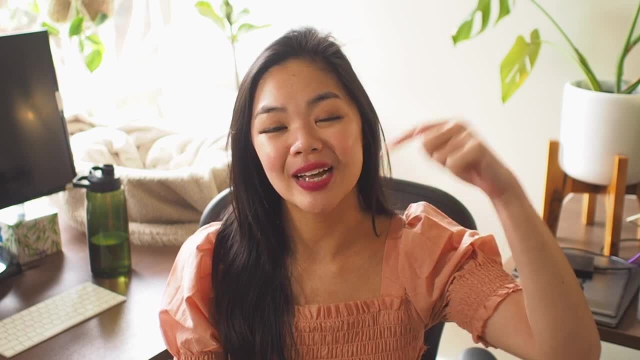 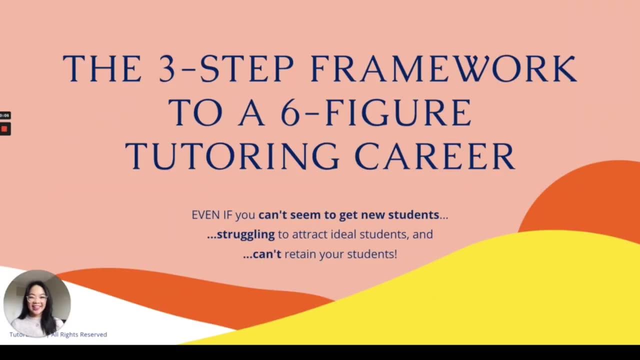 I hope you guys like my quick tip today. Don't forget that my free masterclass is linked in the description below And I'll see you in the next video. Bye-bye. If you're a tutor or you're a tutoring business owner, then you may enjoy that free online.